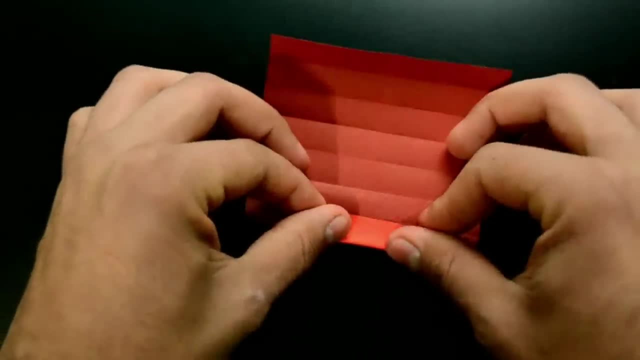 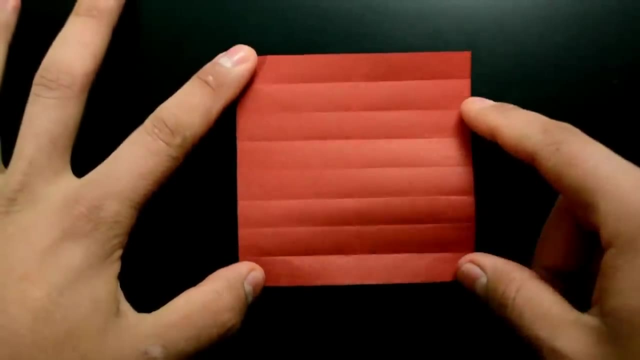 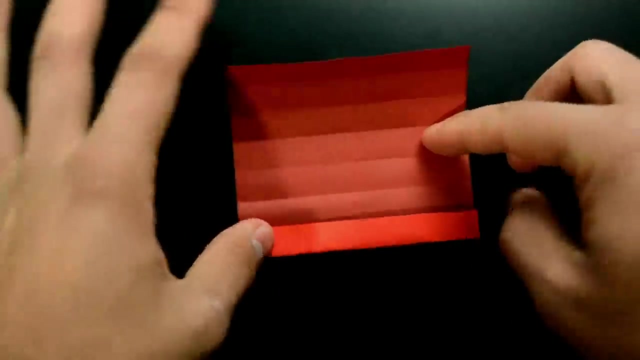 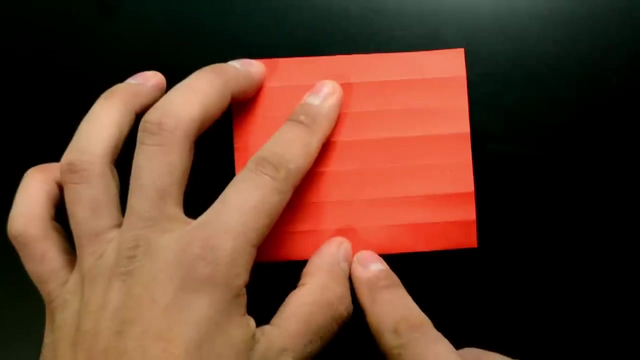 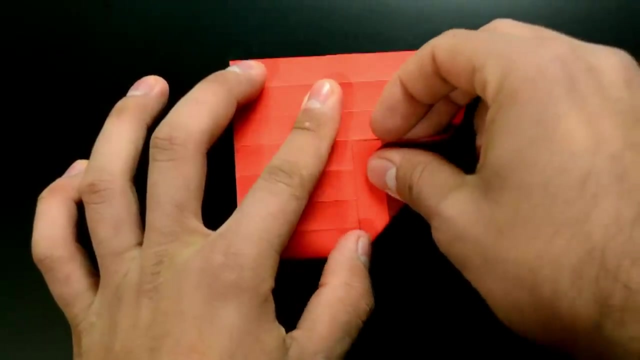 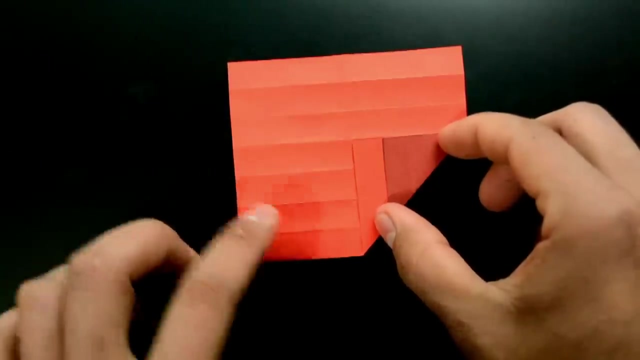 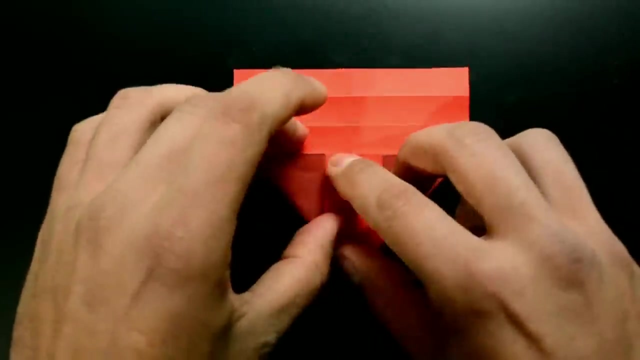 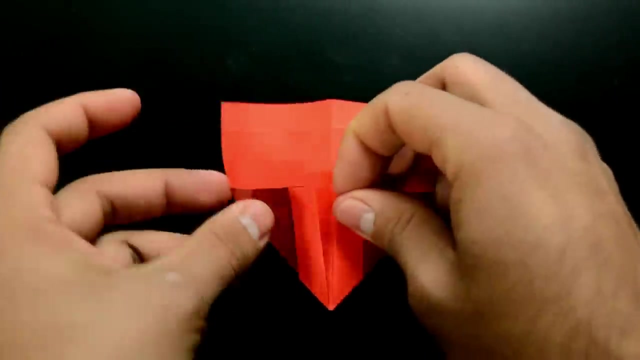 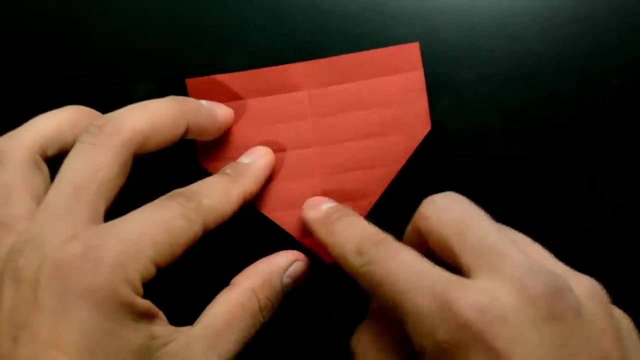 and this step ends like this: okay, we fold only this layer here, the base. turn over and fold this line here, this edge to the middle, creating a new diagonal line in again on the other side. now turn over and fold the bottom corner up using the second crease by. 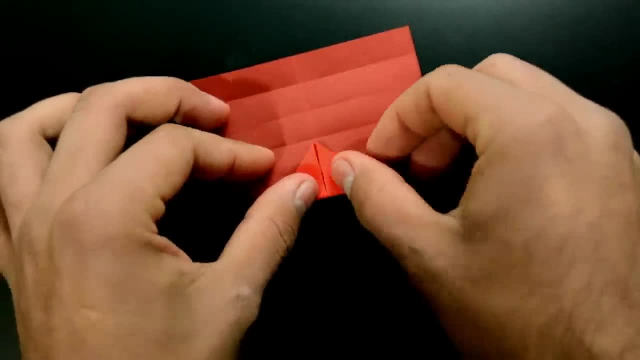 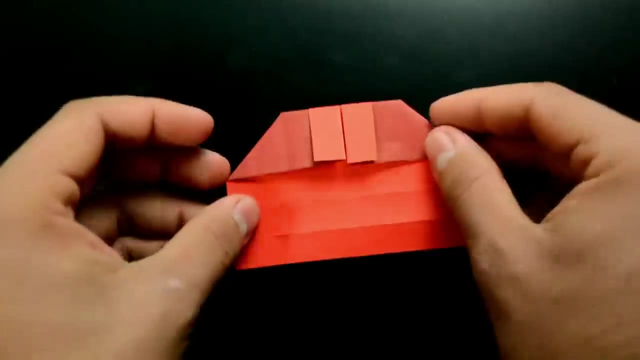 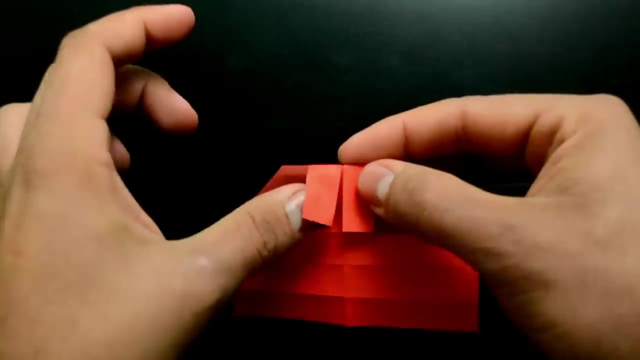 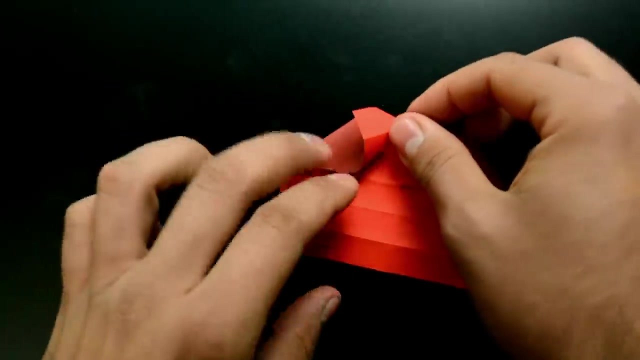 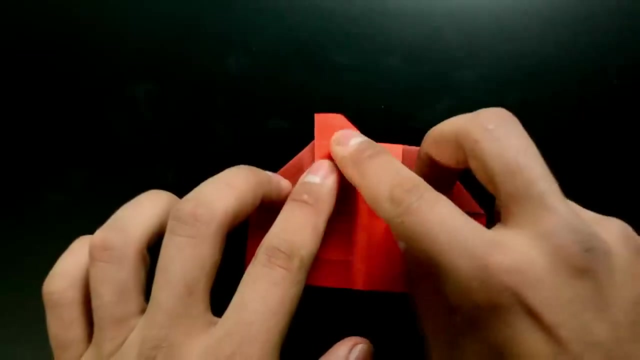 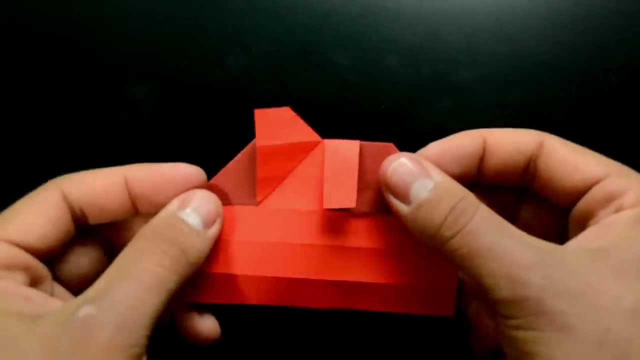 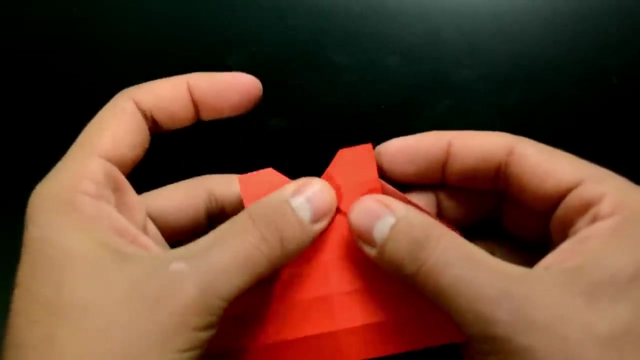 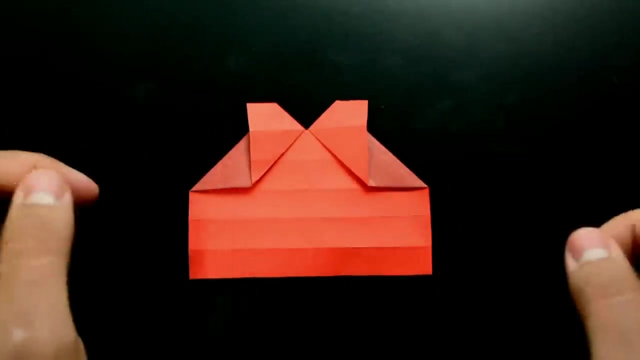 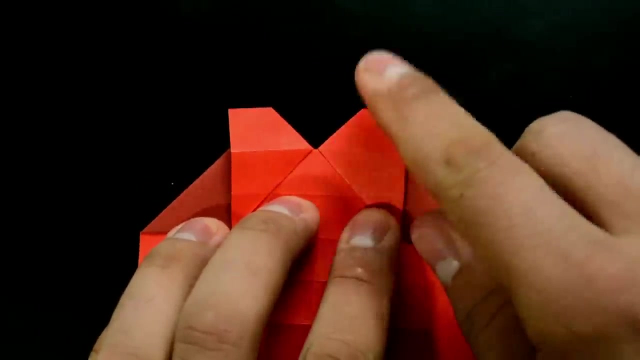 3alterns reference like this: turn over again. now a little attention with the finger: open this layer here like this, and smashing to the top line something like this, and again on the other side. ok, here on the top we have a little diagonal line. we need to fold it in half. 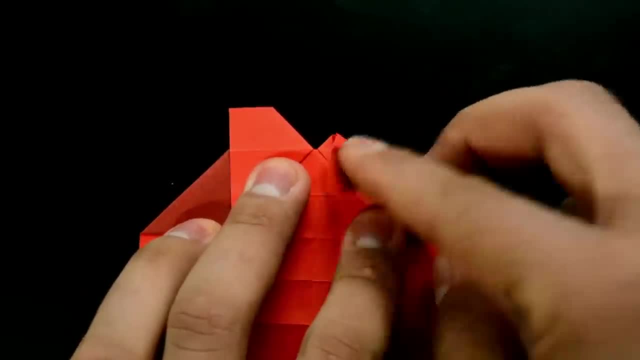 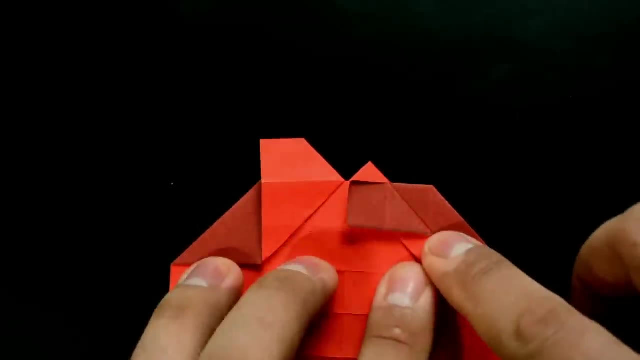 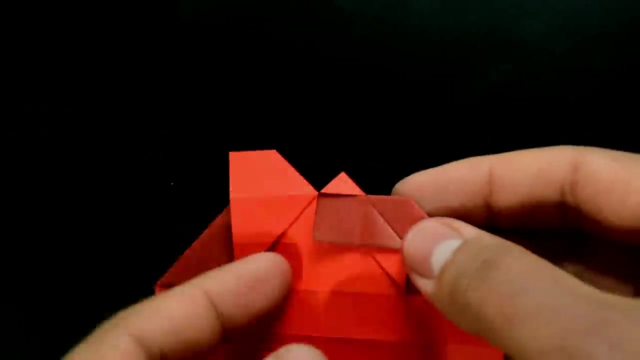 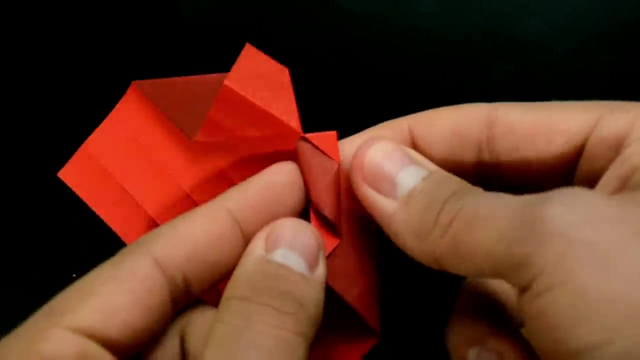 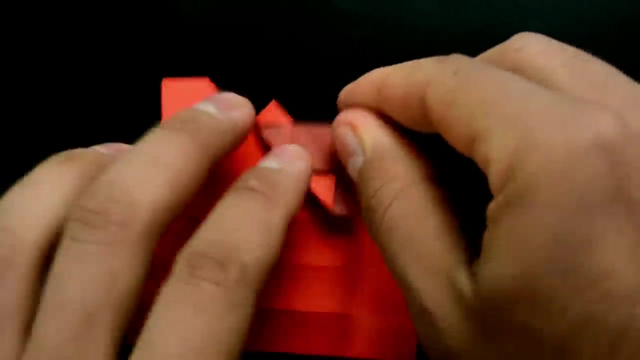 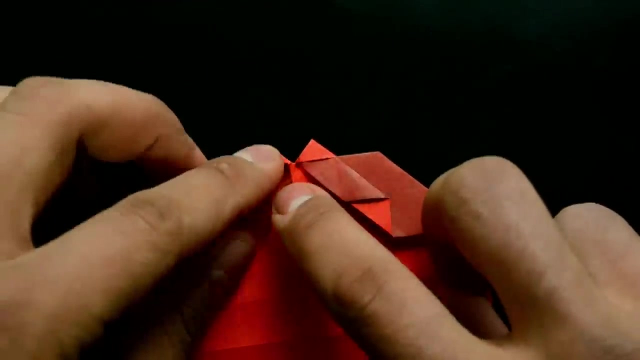 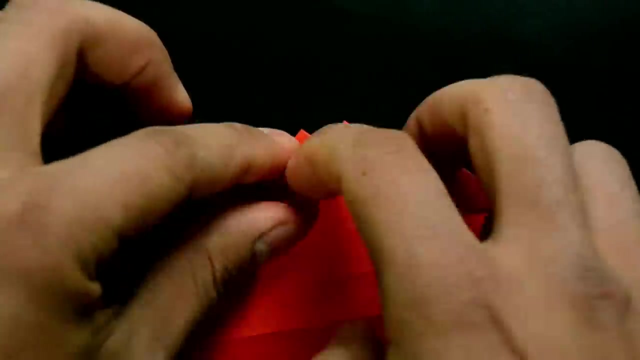 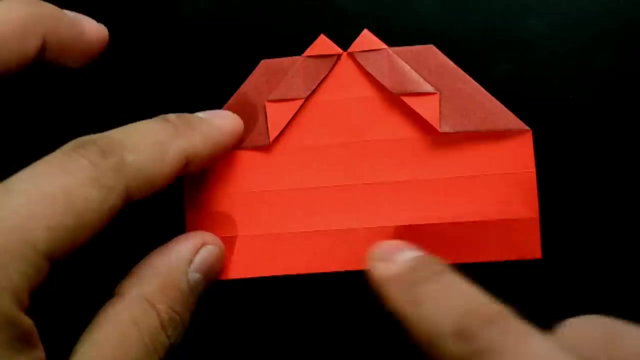 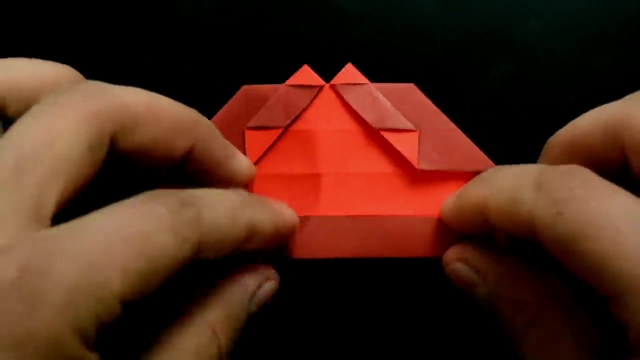 like this and fold this flat. we need to flap this corner here, inside this space here, and repeat this step on the other side. ok, to the next step. we need to fold this layer here like this, and again the same step until the end.